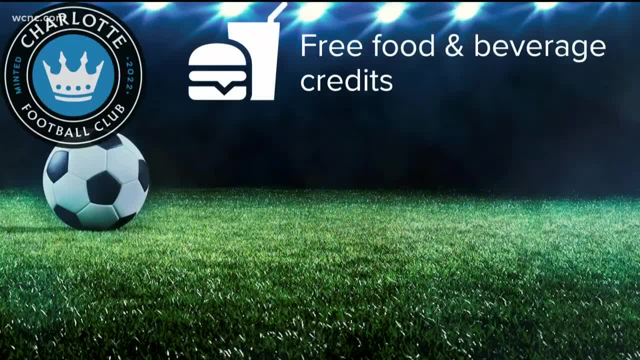 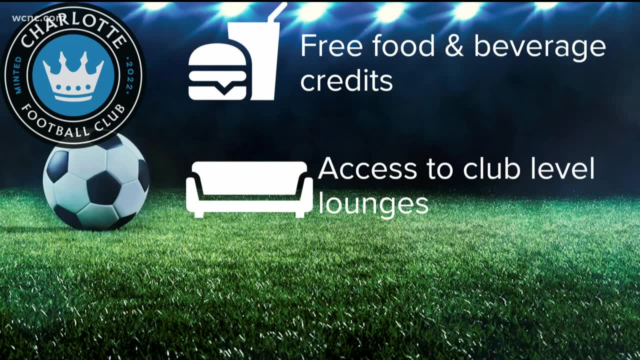 you'll be paying extra. Charlotte Football Club says that part of the reason the prices are so high is because you get perks of see. you get access to club level lounges, free food and beverage credits for every game. Carolina Panthers- Charlotte Hornets.